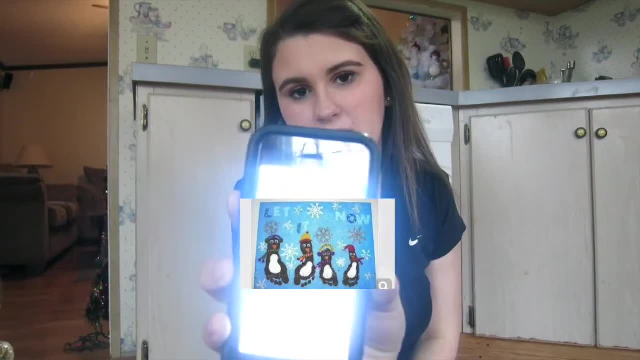 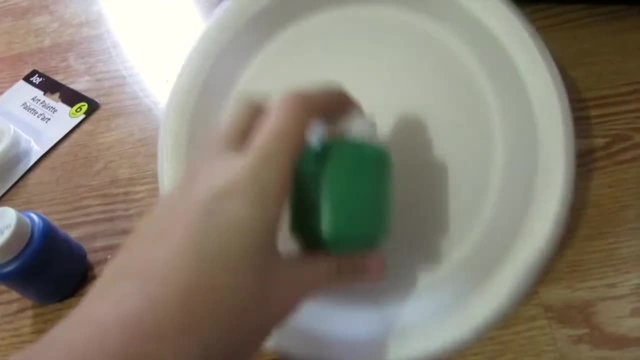 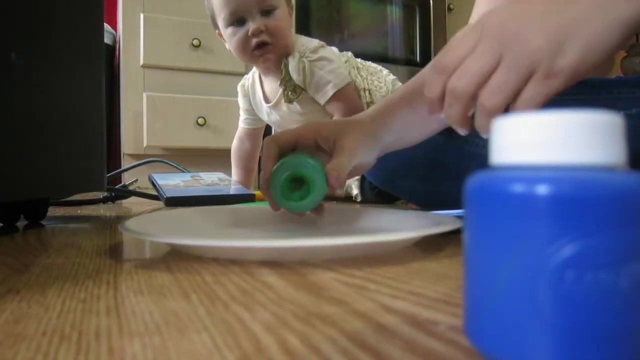 I'm trying to accomplish Penguin, a Christmas penguin and a Christmas tree. Alright, so I'm going to take the green and I'm going to put it on this paper plate so I can accomplish this tree. So we have our green paints. 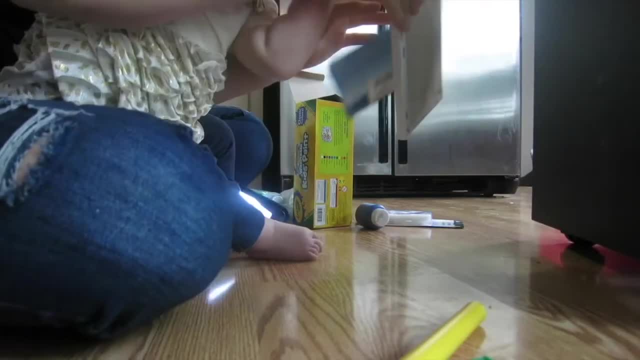 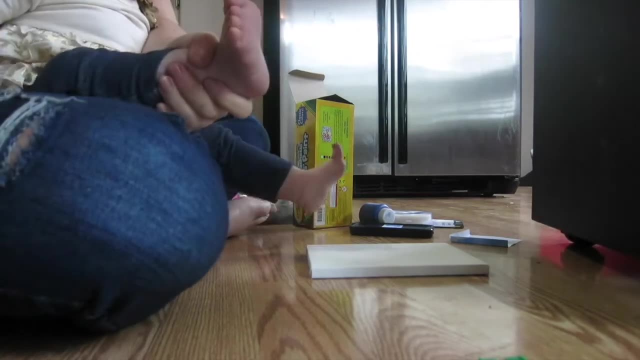 And I'm going to put it on her foot now. Hand this up, first of all. Alright, so I got the canvas open and now I'm just going to put her foot in the paint and see what happens. I actually might just rub it on her foot. 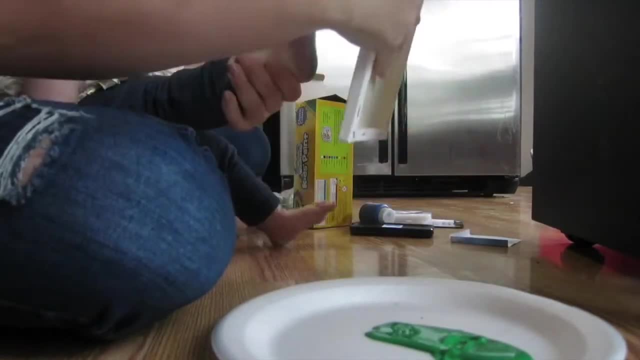 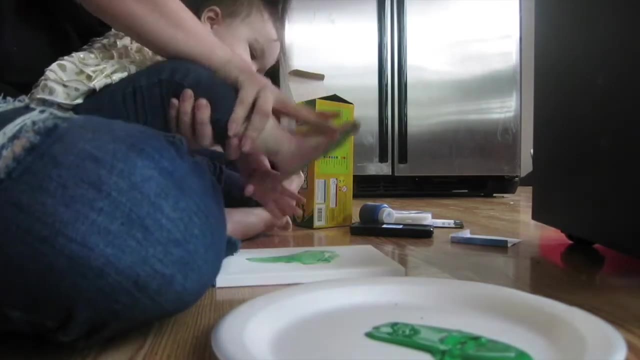 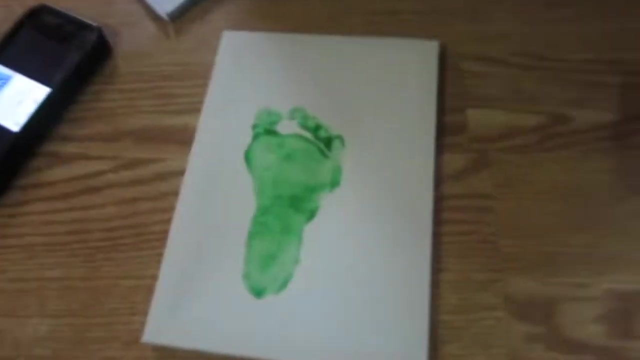 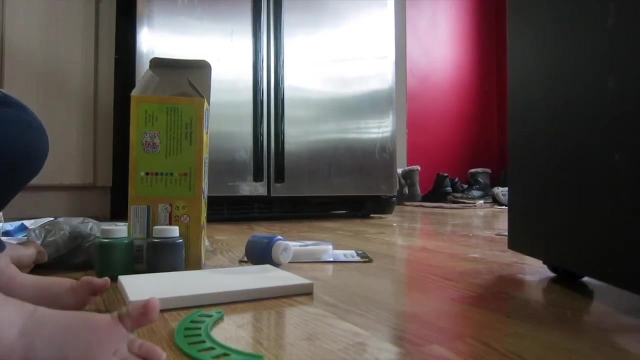 Alright, so now I'm going to try to put her foot on it. oh my gosh. okay, I don't know how much of that I recorded, but it turned out cute. I did it. alright, so now we're gonna do the black footprint for the penguin I have. 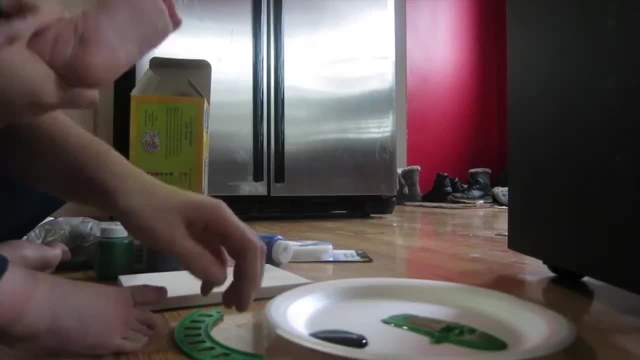 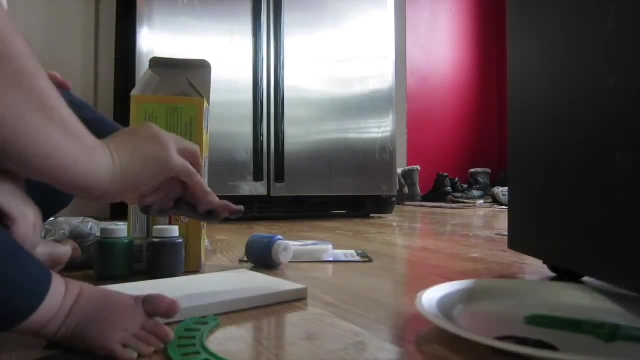 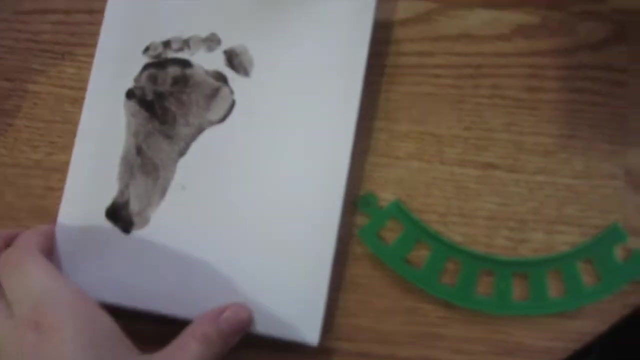 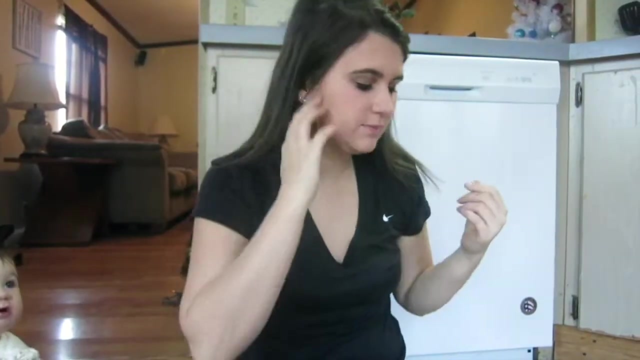 our black paint. okay, guys, I'm actually really excited because these are turning out not as bad as I thought they would. I mean it's not a perfect footprint, but I mean it's not bad either. so, honestly, at this point I think I'm gonna attempt the mistletoe one. 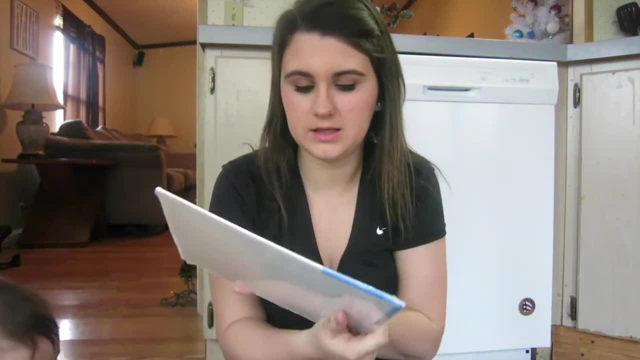 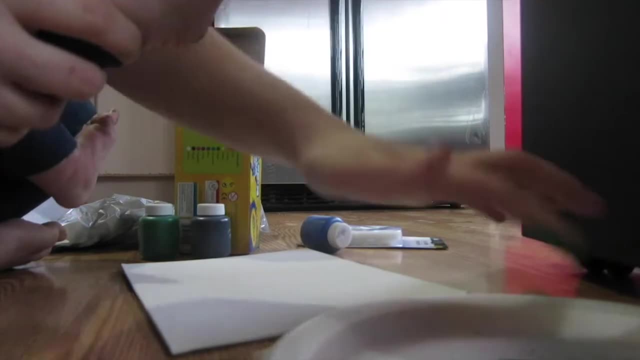 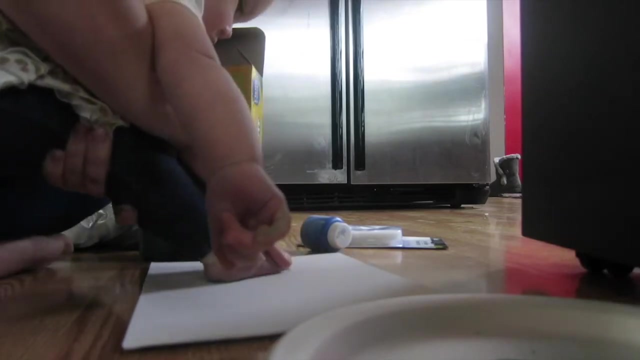 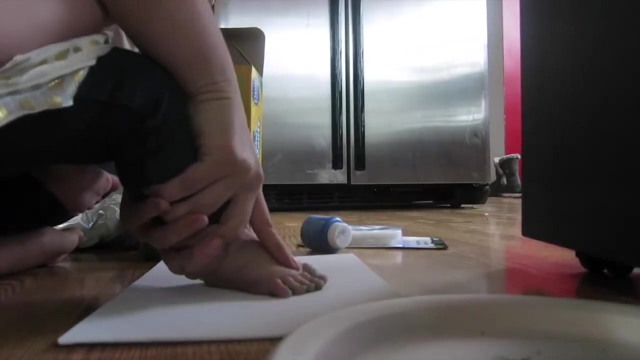 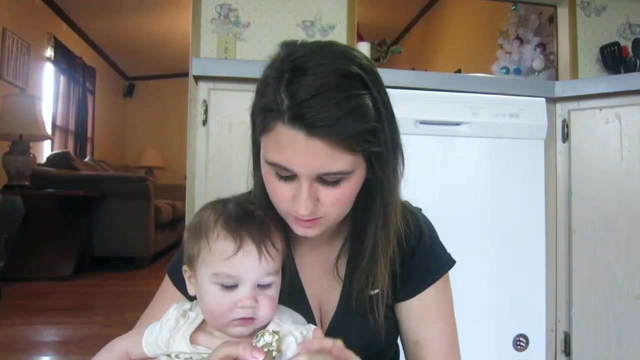 with her feet and just put it on the ground, and then I'm just gonna put the Put it on the big one and see if I get lucky on that one too. So this turned out really good. I'm about to show you what it's supposed to look like. 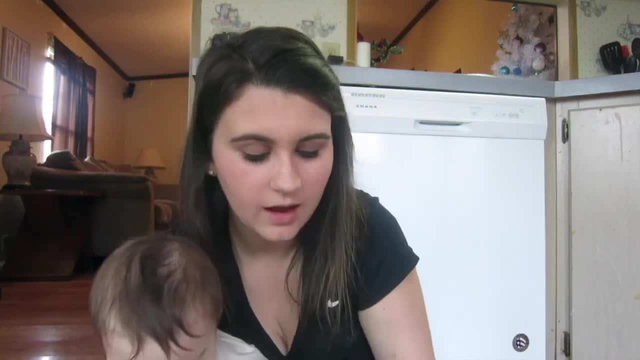 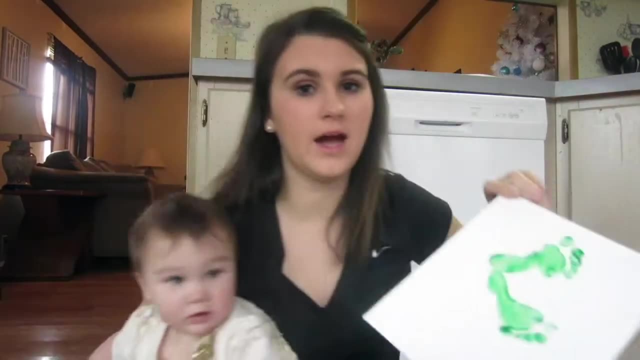 Hopefully you can see that, but I mean I did pretty good. I think It's a little crooked, but I'm pretty excited. So when these are done drying, I will show you how we're going to paint them and get them ready for being presents. 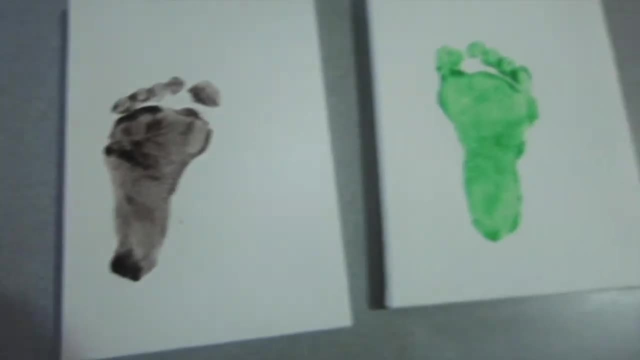 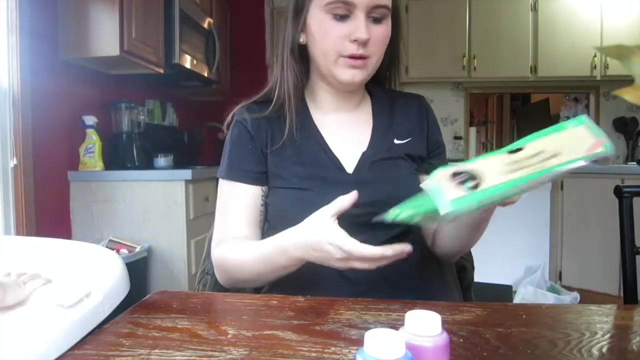 Oh, we did so good. So while those are drying, I thought I'd be able to show you guys what I did. So while those are drying, I thought I'd be able to show you guys what I did. So while those are drying, I thought I'd be able to show you guys what I did. 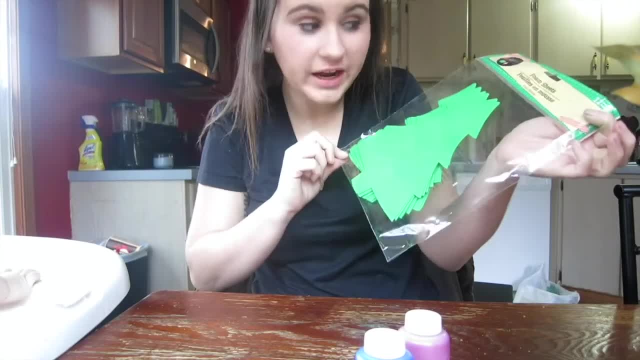 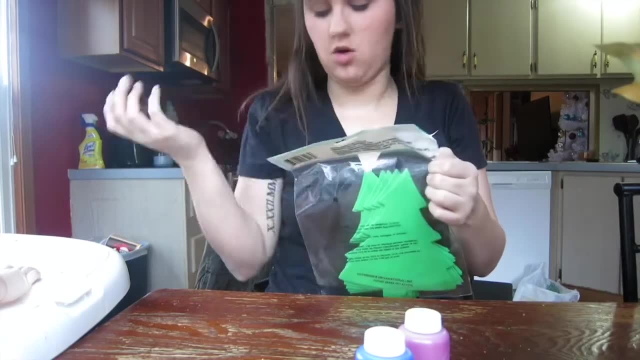 I'm going to be really brave and try to let her paint a Christmas tree. This is probably a bad idea and this is probably where it goes bad, but oh well, We're going to do it anyway. So I got these at the Dollar Tree. 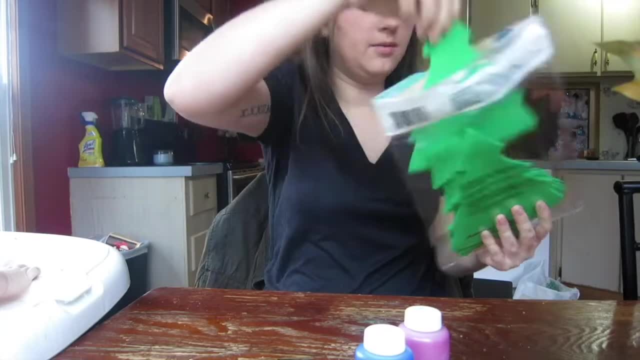 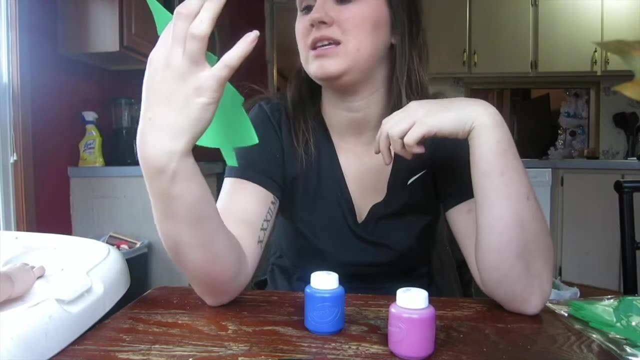 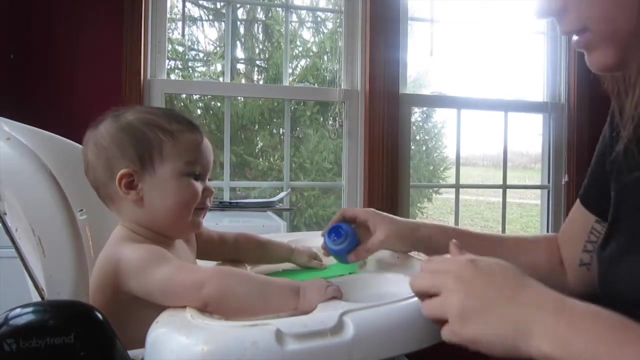 It comes with 12 of them, So deal. It's just a foam Christmas tree and I got two colors. I'm going to attempt to let her paint it and see how that goes. Let's see here. okay, I'm going to put a little bit of blue right here. 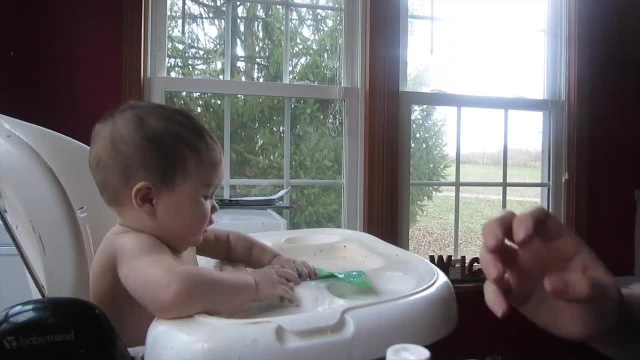 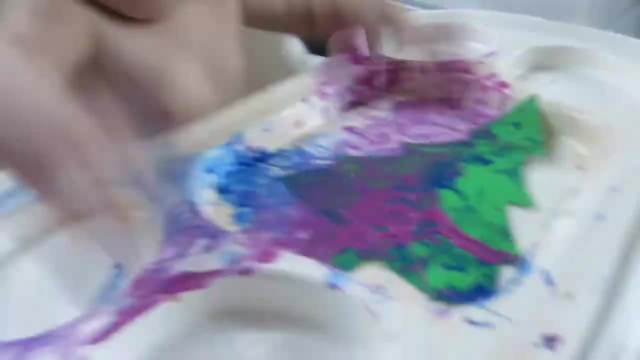 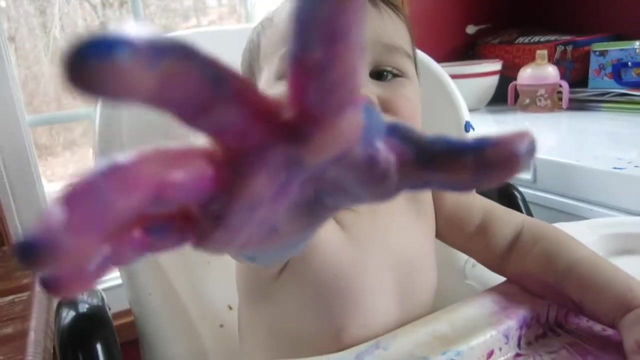 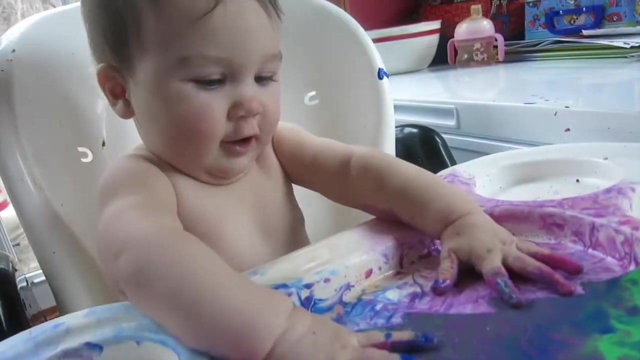 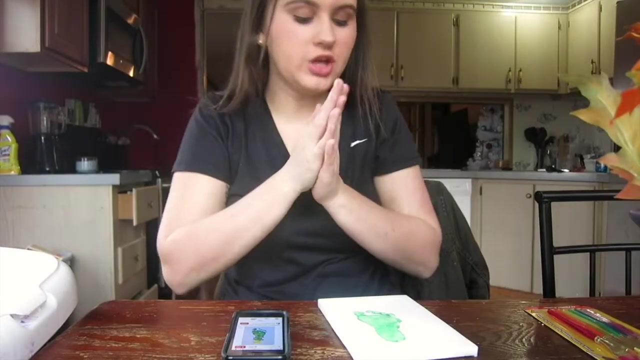 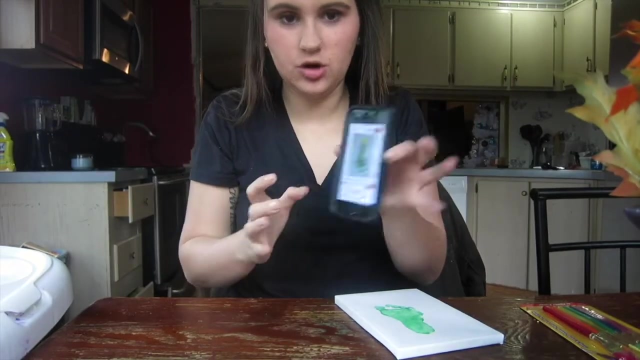 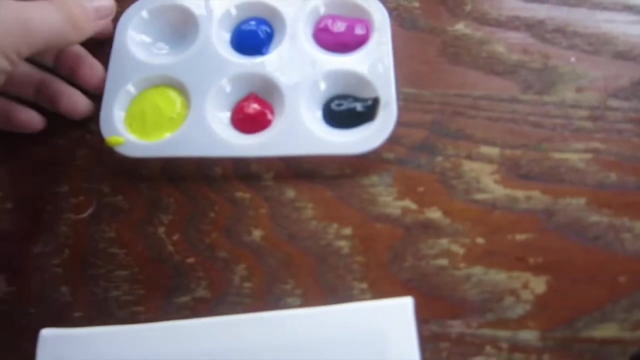 I'm going to put a little bit of blue right here, So the first green footprint is pretty much dry. so I'm going to start making it look like a little Christmas tree, and so I have my setup right here. I have my paint in this little thing, I have my paint brushes and what it's supposed to. 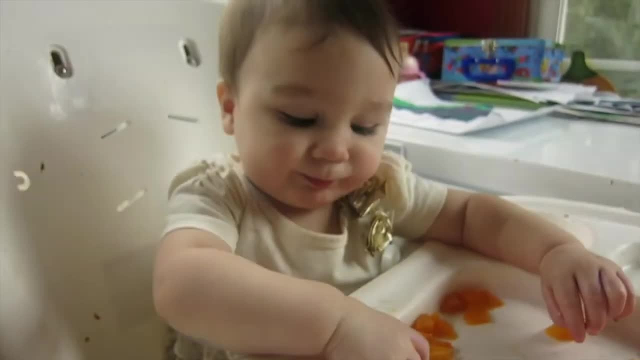 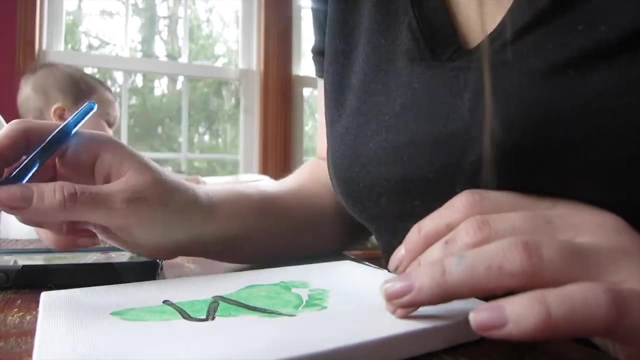 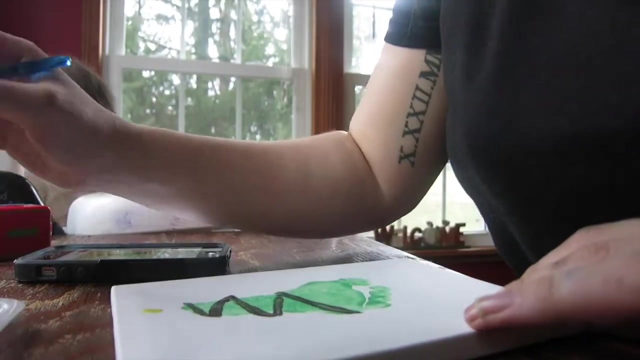 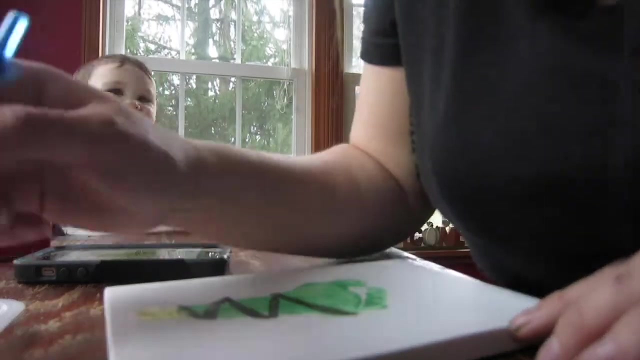 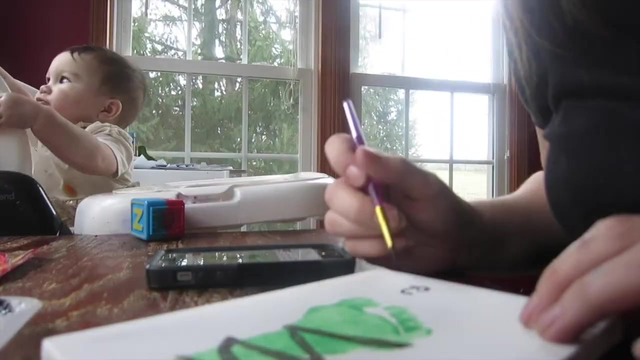 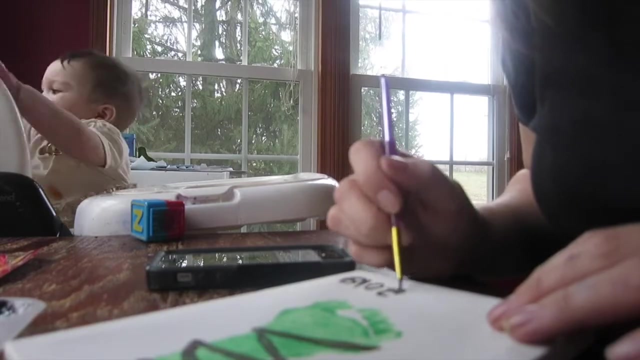 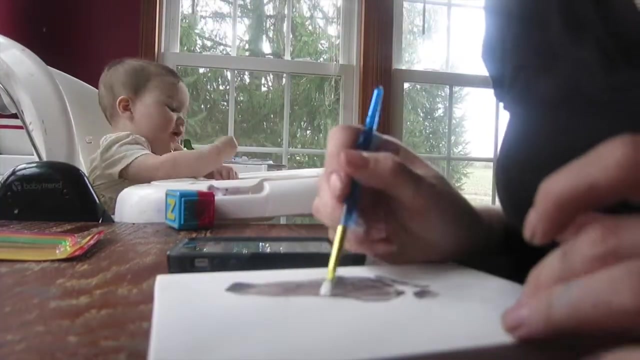 look like A little helper. she's all cleaned up now and she's eating some peaches, So I'm going to take my guess and I'm going to try to make it look a little bit more like a little tree. There we go. 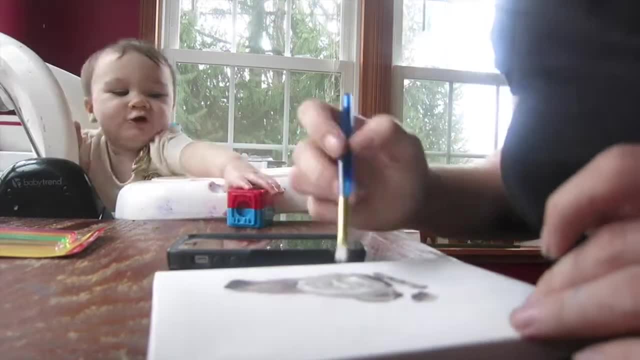 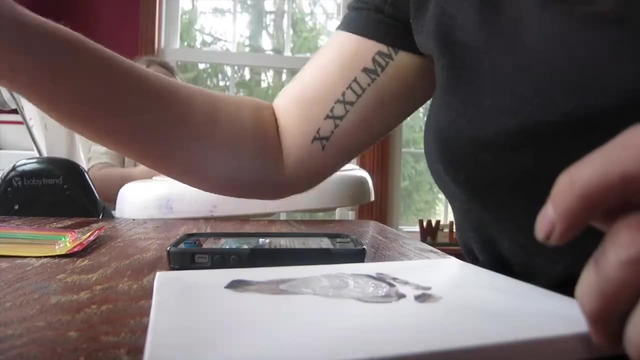 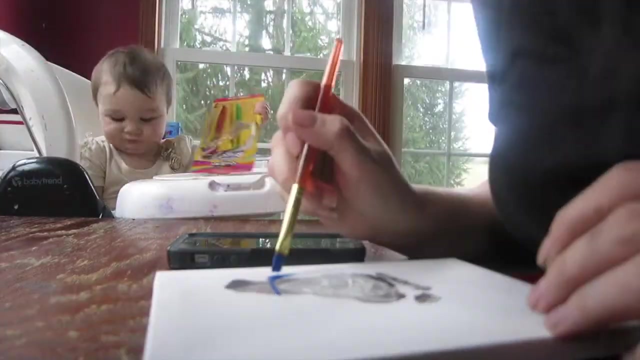 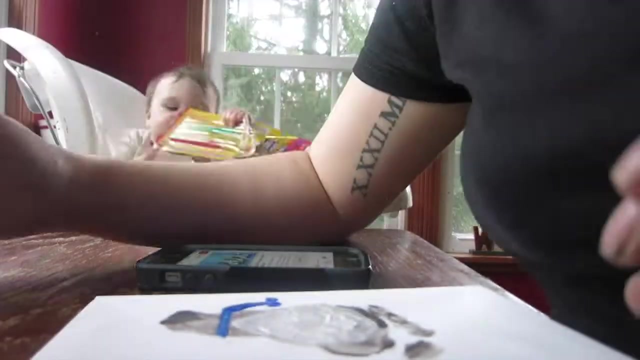 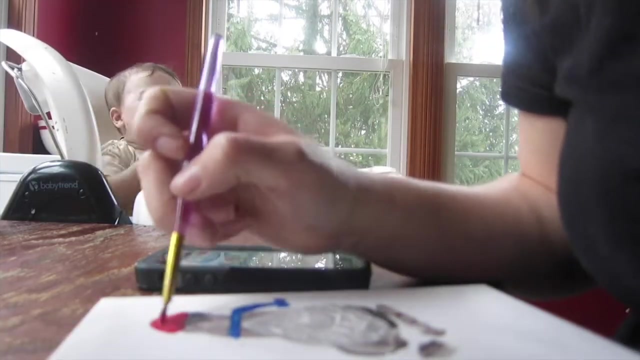 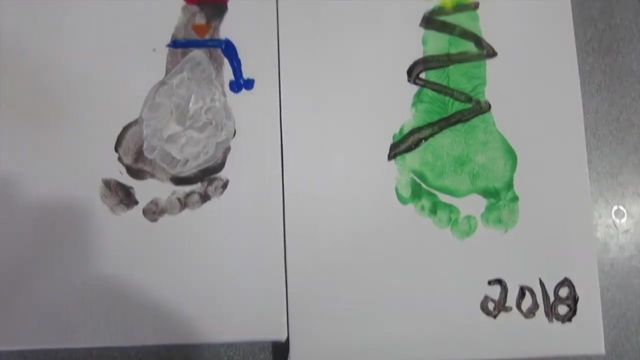 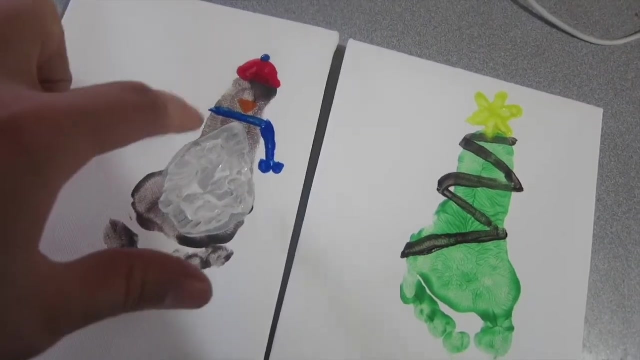 Alright, so I'm going to start with the middle. I don't want to get it too small. Alright, there we go. Alright, This one's still drying and this one's still drying. I've got to put the googly eyes on this one and put the stripes on his scarf and he'll be done. 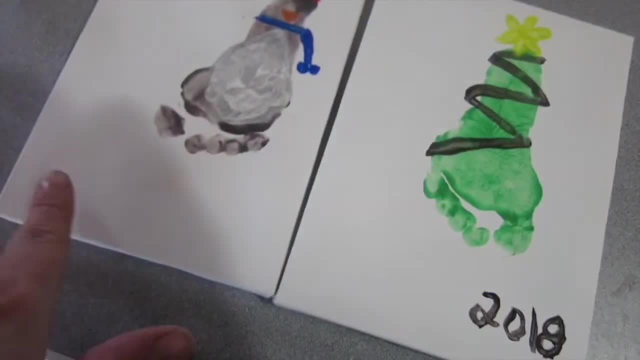 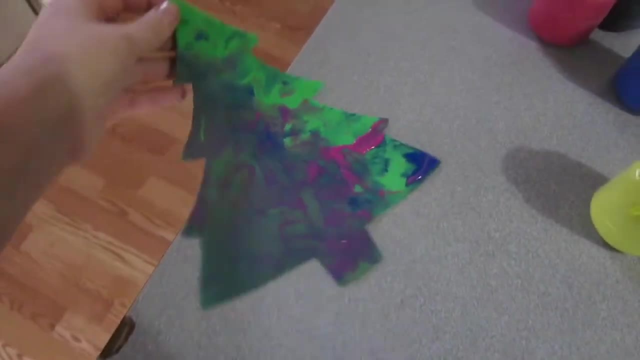 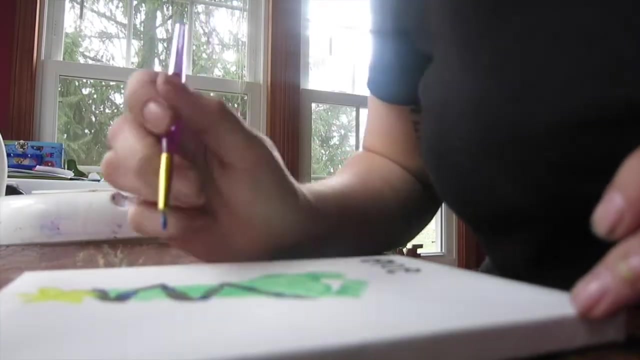 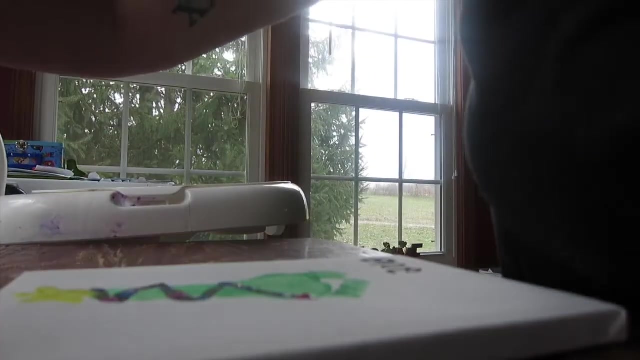 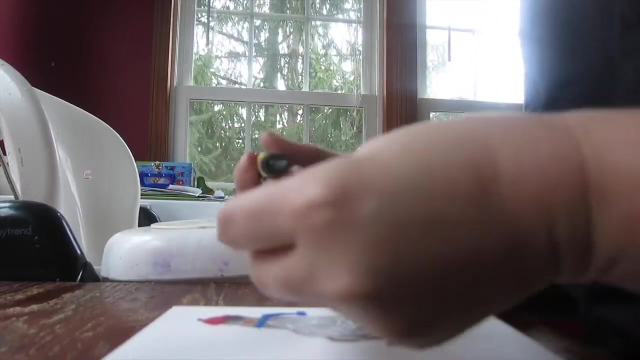 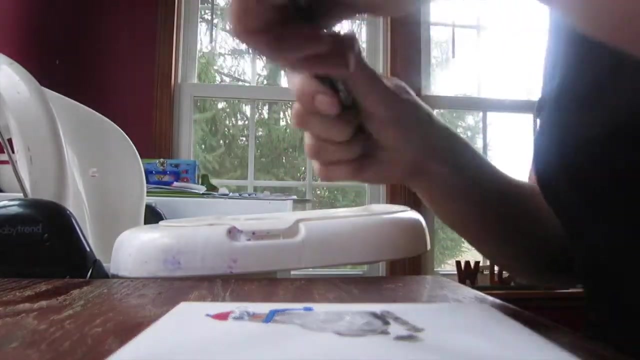 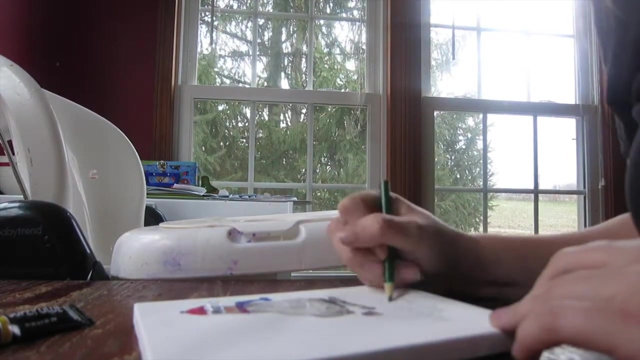 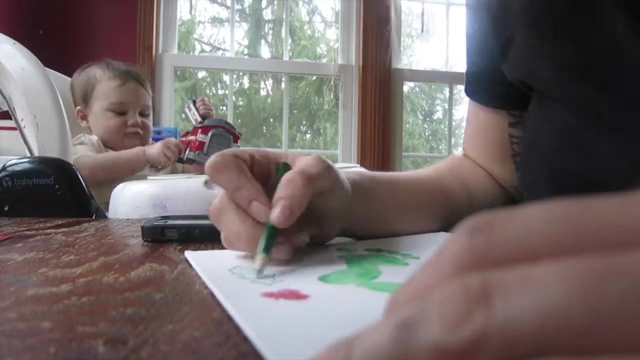 And then this one: I've got to do the little Christmas lights And I've got to write 2018, Addison Marie on these, And this is her beautiful tree that she painted as well. And this is her beautiful tree that she painted as well. 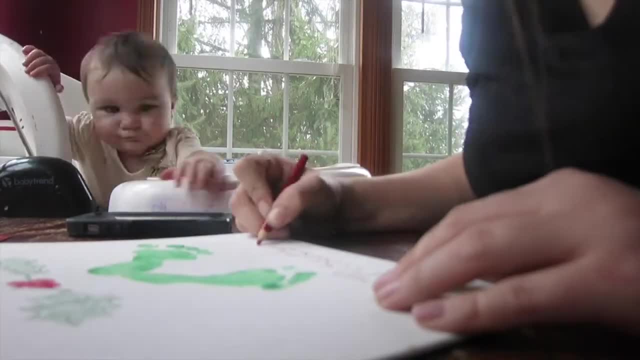 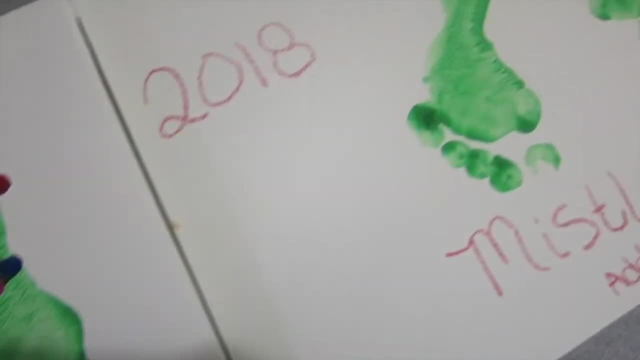 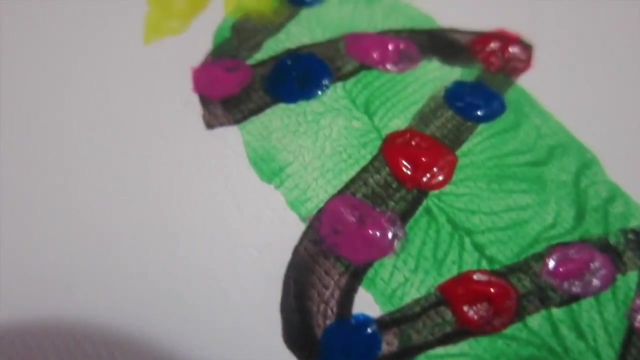 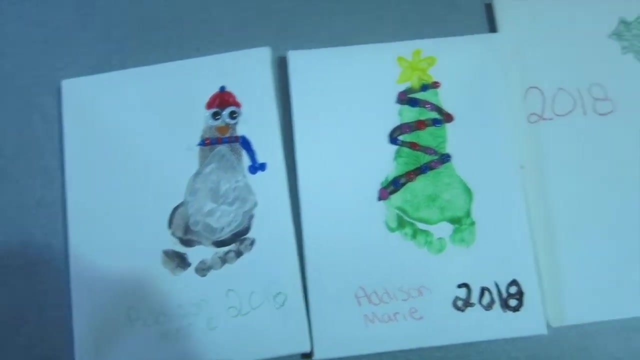 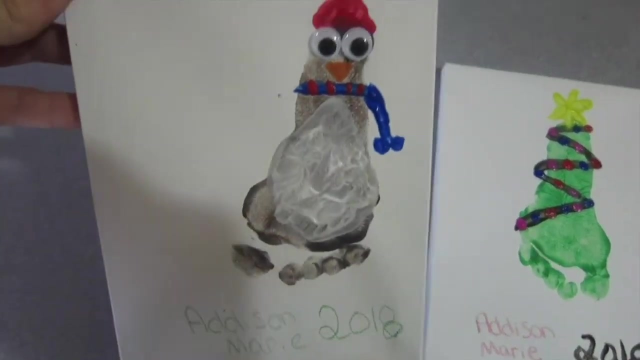 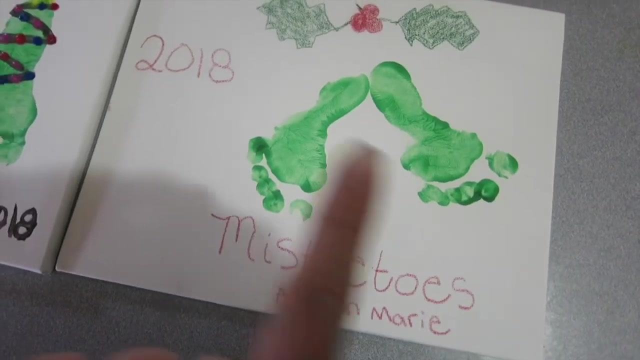 Okay, you guys. so they are done and I'm so excited They turned out so cute. Here's the penguin: I just super glued his eyes down, so he's still drying. Here's the Christmas tree And here is the mistletoes. 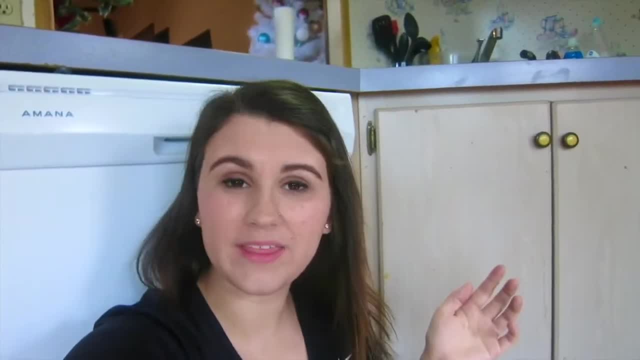 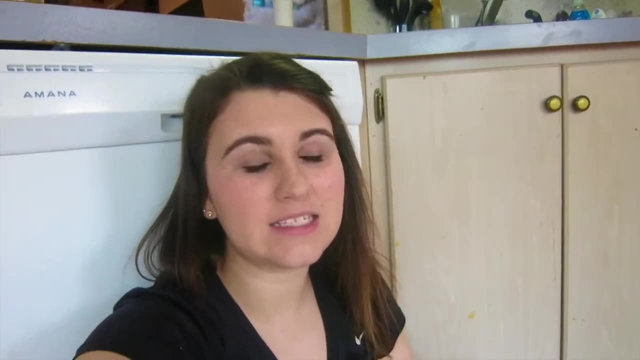 They're so cute. Alright, guys, so I hope you enjoyed that video. Some Christmas craft ideas for babies. These are perfect for gifts from the kids. And stay tuned for next week, because next week we're going to do preschool crafts for Christmas as well. 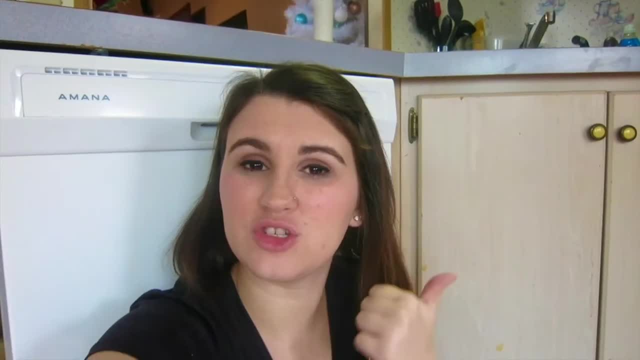 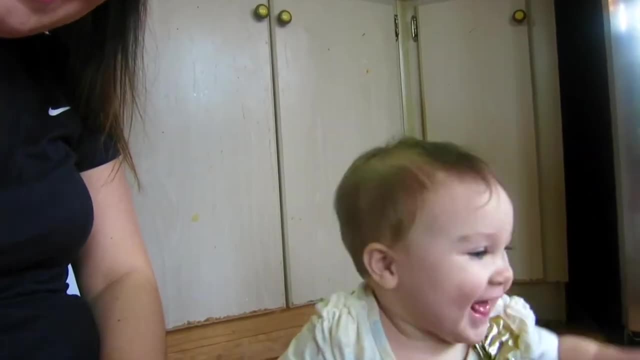 So I hope you guys enjoyed. If you did, please give it a big thumbs up and subscribe And let me know in the comments. Say bye, guys. Say bye. One of these days she's going to say bye, I promise.